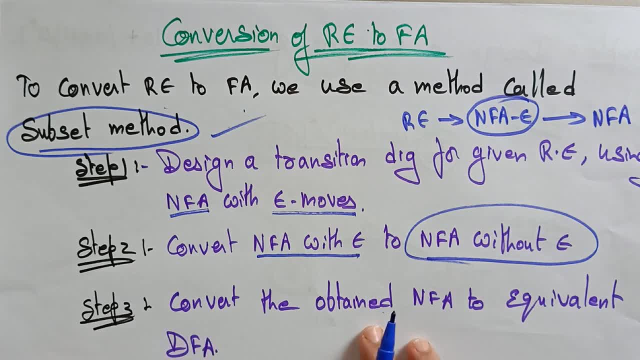 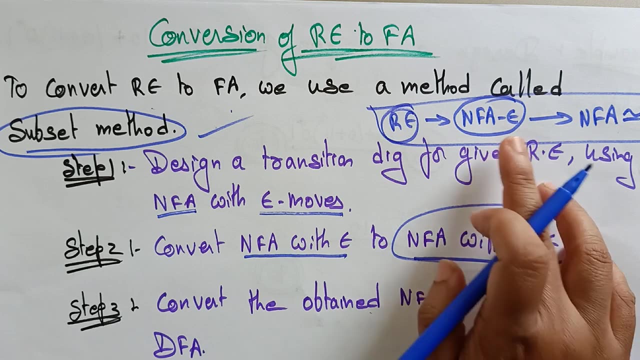 finite automata. So finally, convert the obtained NFA to equivalent DFA. So for this, you need to convert the equivalent DFA. So these are the steps that you need to be follow. Okay, first, take the regular expression: convert into non-deterministic finite automata with epsilon modes. So after that, 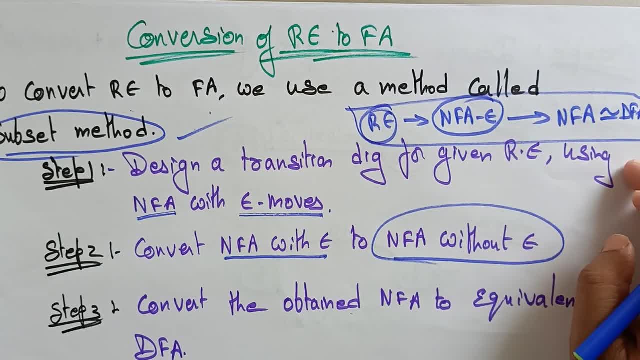 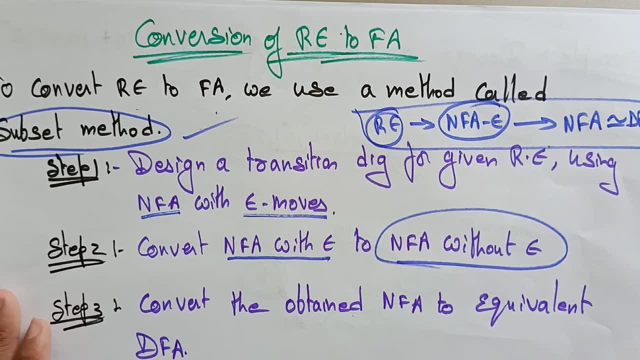 remove the epsilon modes and means, you will get the NFA. Finally, you have to construct an equivalent DFA for the given, for the whatever the NFA we get. Okay, so let's see the example, Then you can clearly understand how we are going to convert. 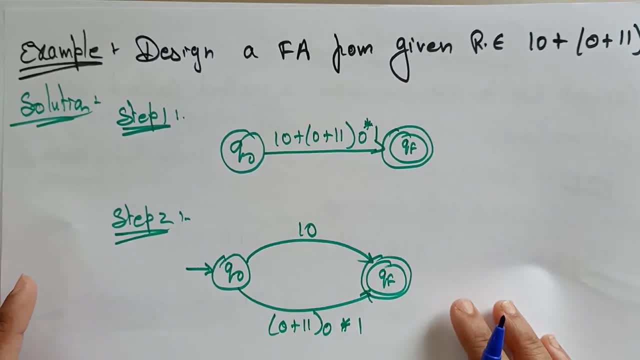 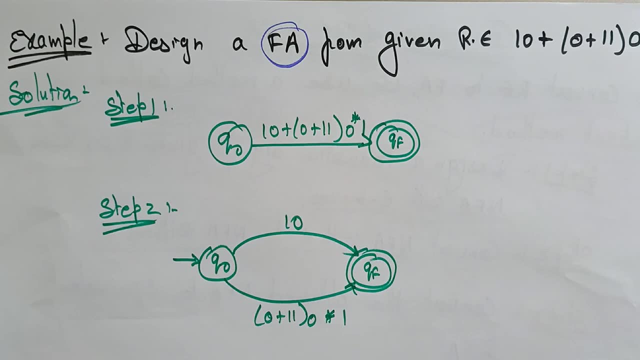 from regular expression to the finite automata right. So here I have taken an example: design a finite automata. So I need to design a finite automata, whether it is a non-deterministic finite automata or deterministic finite automata from a given regular expression. So this is a 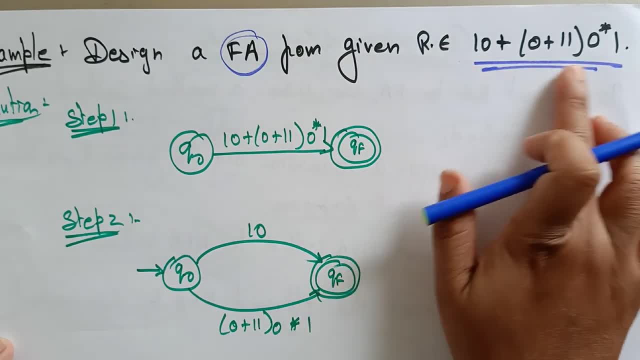 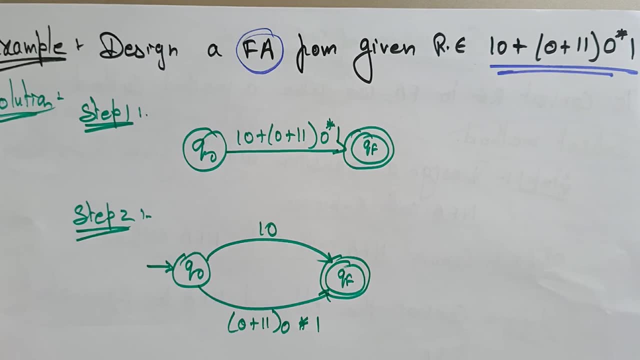 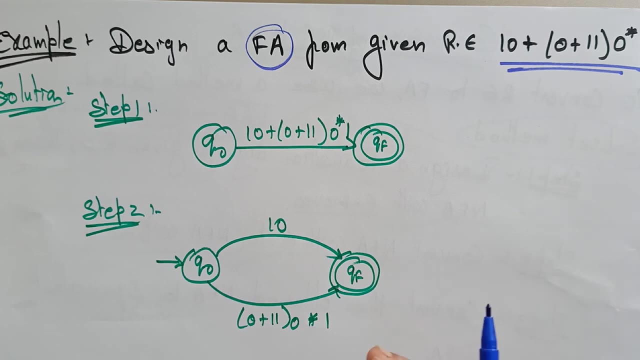 representation of regular expression. Okay, so this is a representation of regular expression. Now let's see. First step is what is the first step? What I said? First, I need to convert the regular expression into non-deterministic finite automata with epsilon modes. After that I have to remove the epsilon. 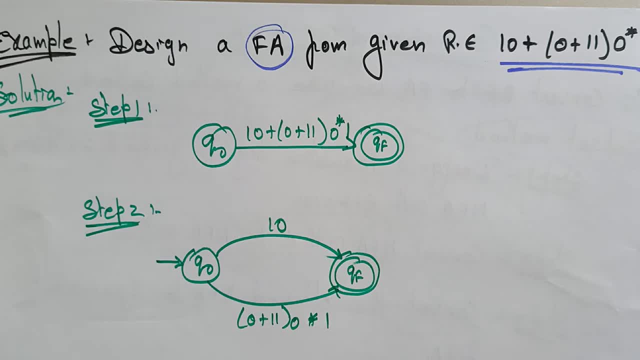 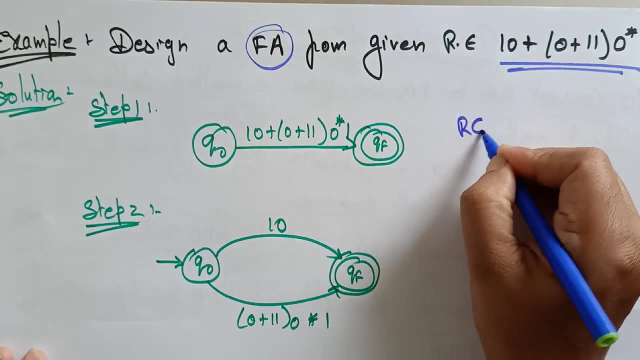 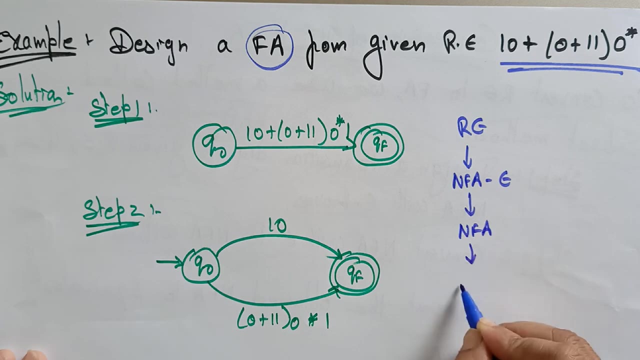 modes and make it as a non-deterministic finite automata without epsilon. After that I have to convert into equivalent deterministic finite automata. Okay, so regular expression to NFA with epsilon modes. Next you have to convert it into NFA. After that DFA. 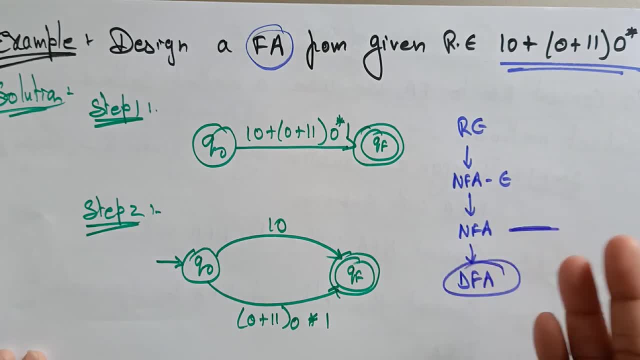 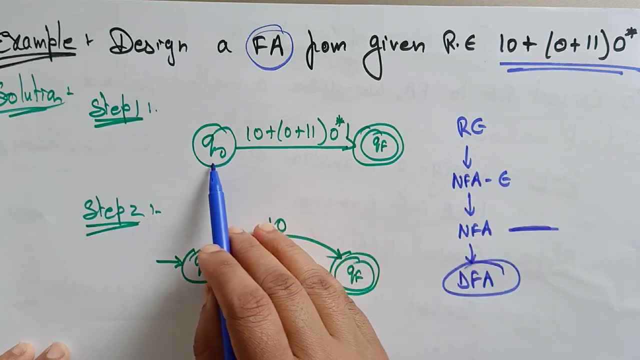 If you want, you can convert into DFA, Otherwise you can stop here, because non-deterministic finite automata is also a finite automata right. So first step, the regular expression I can. I represented in the transition diagram. So. 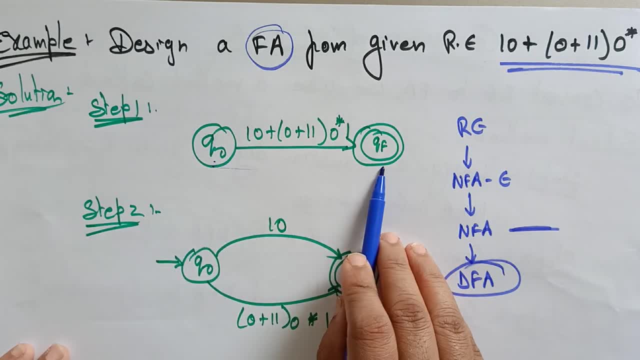 I have taken. initially, I have taken Q0 as initial state and QF is a final state. Because this is a finite automata, there should be an initial as well as the final states. Okay, so I just represent whatever the regular expression that is there. Q0 is ending that. 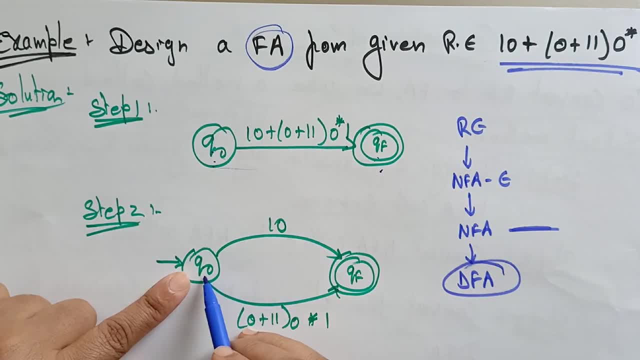 expression to the final state. Now split this, The Q0,. I am splitting this into two because the plus is there. So 1, 0 is going to the final and 0 plus 1, 1, 0 star 1 going to the final state. 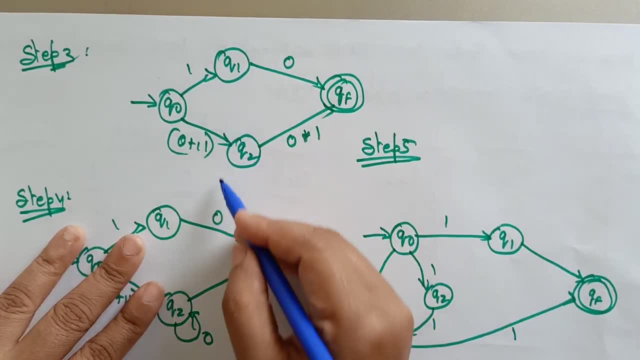 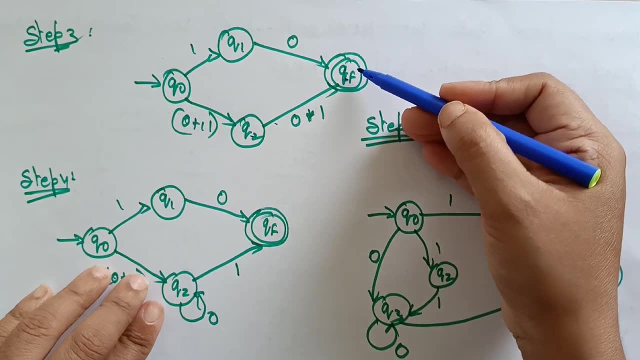 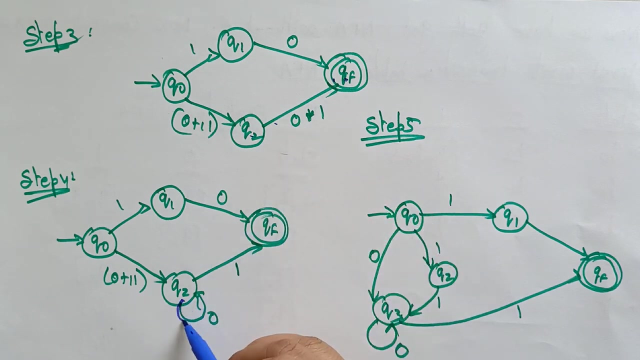 So next step, again split. Okay, so again split into two parts. So 0 plus 1, 1, Q1 and Q0, and everything should reach us to the final state. The final expression should reach to the final state. And step 4, again divided. So here the 0 star is there. So 0 star means 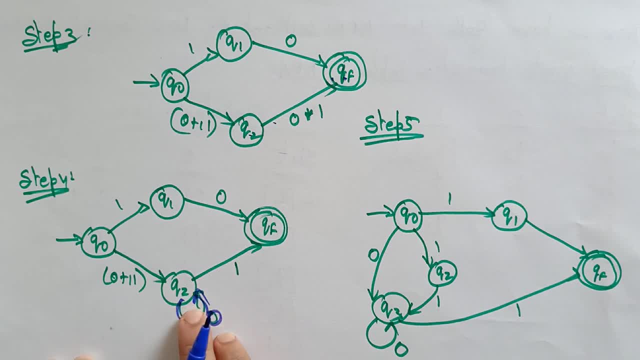 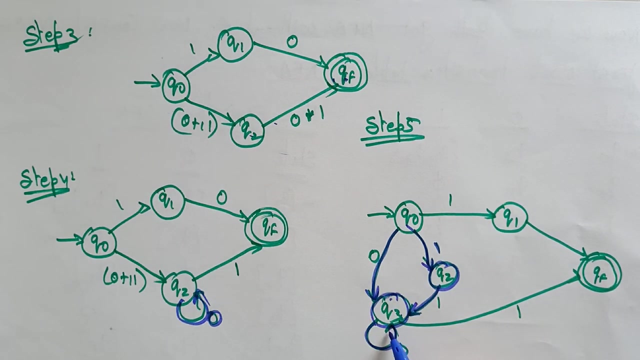 a loop will be there, So it will be connected to the Q2.. Okay, again, 0 plus 1 has to be divided into 0, 1, and take an intimate Q2 and another state Q3.. Now the loop is 0, star is. 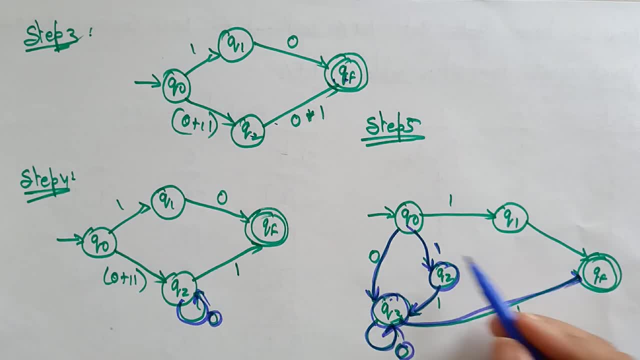 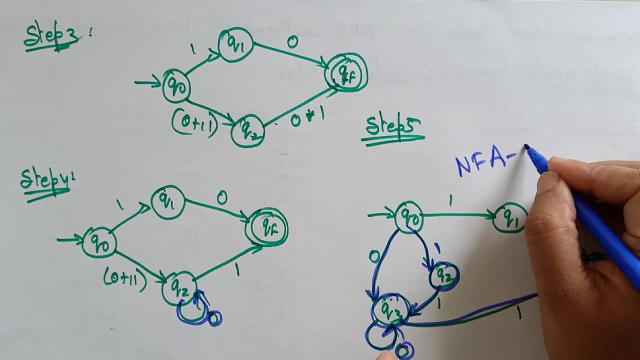 connected to the Q3 and Q3 is connected to the Q4.. Okay, So this is how you are going to design a transition diagram. So this is an NFA transition diagram. So regular expression is converted into NFA transition diagram without epsilon. 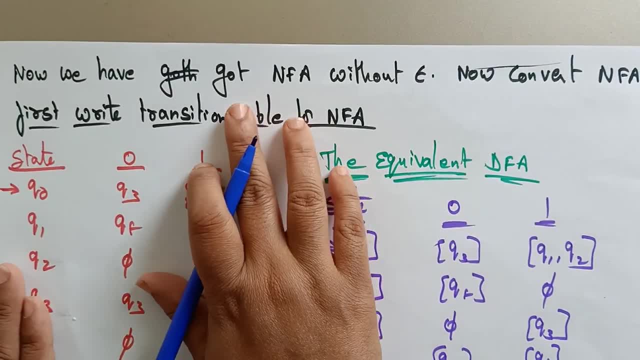 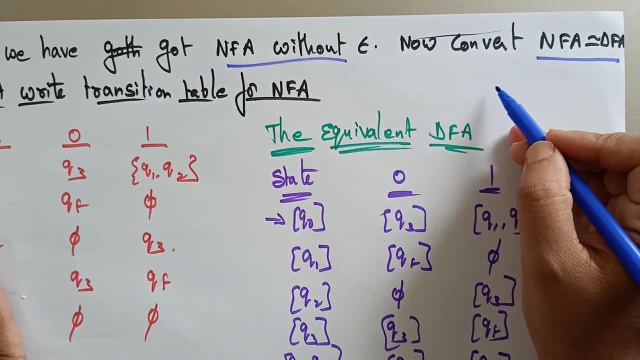 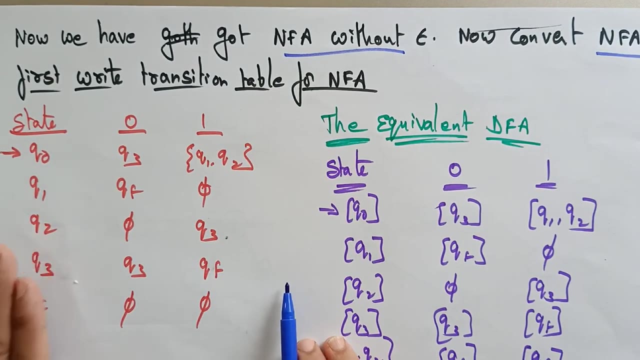 So next we have got NFA without epsilon moles. So now convert NFA to the equivalent DFA. So that is a concept, right. So I have to convert the NFA into the equivalent deterministic finite automata. First write the transition table for the NFA, whatever I got. So this: 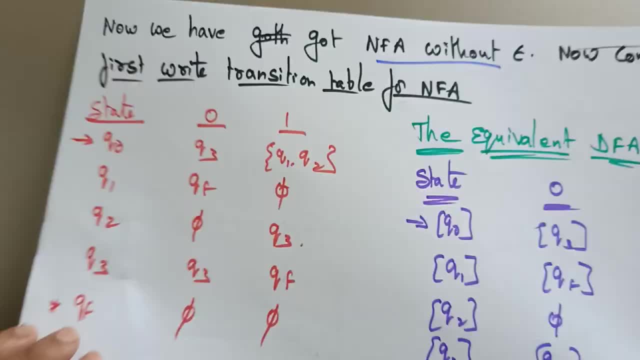 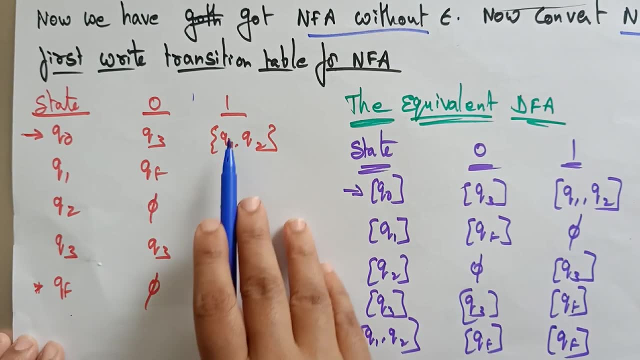 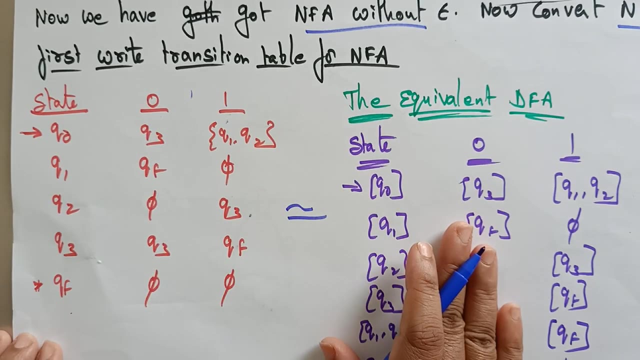 is the transition diagram I got By seeing this diagram I converted. I represent the transition table. Q0 is initial state and QF is the final state, And these are the next states for the given input. Okay, Now I am going to convert this to the equivalent deterministic. 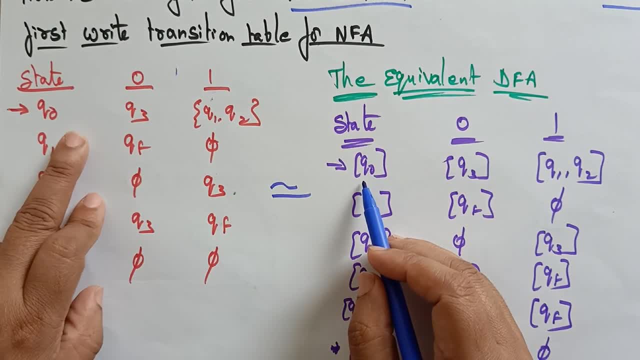 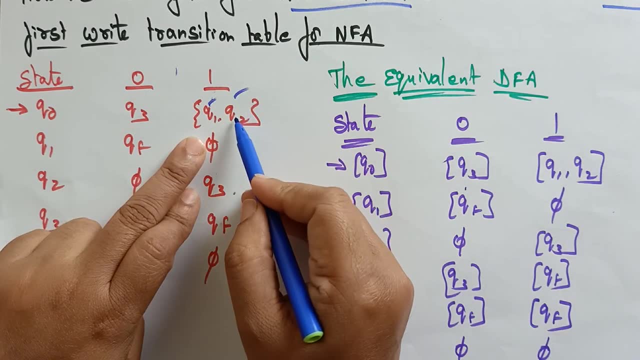 finite automata. How? Let's see Q0, the next states on 0 is Q3 and I am taking Q1 and Q2.. These actually in NFA these are the two separate state, But in DFA both becomes a single state. 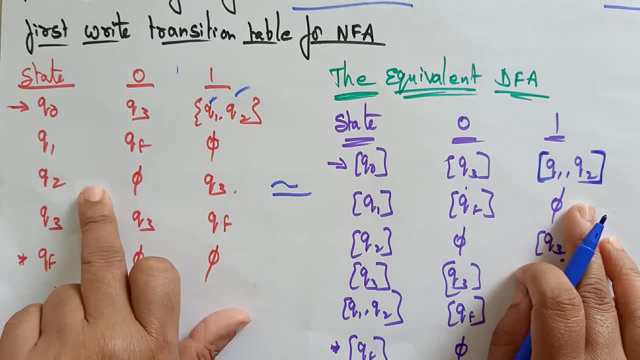 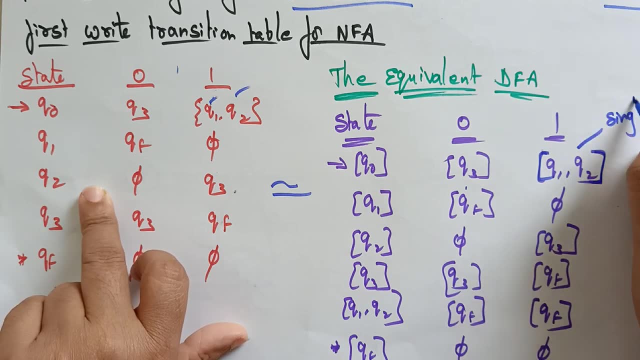 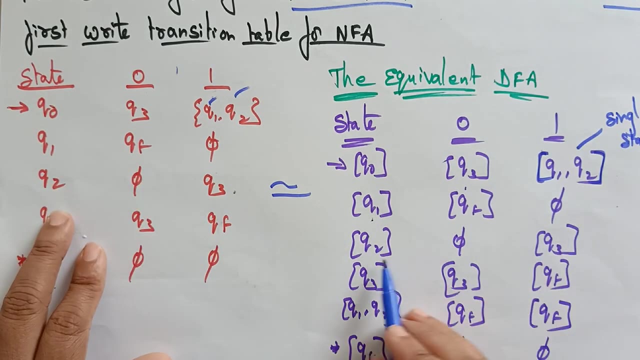 So here Q1 and Q2 are separate states in non-deterministic finite automata, Whereas in the deterministic finite automata they are together called as a single state, Single state. Okay, Now take the Q1, Q1, QF, Q5, empty string, So Q2, I represent Now Q3,. 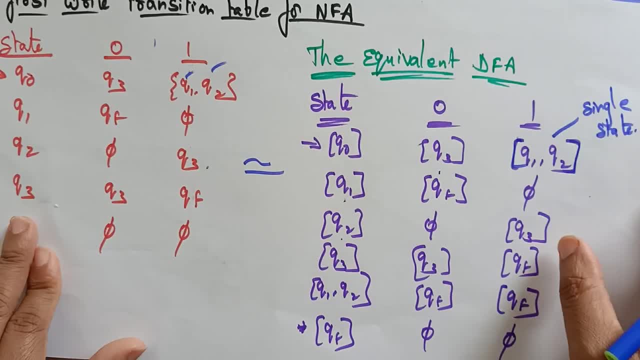 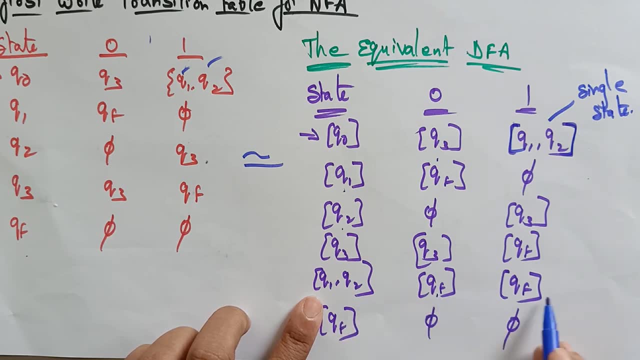 represent Now the new state that we got. it is the Q1, Q2.. So this will be the new state: Q1, Q2.. So the Q1, Q2 will reach us to the final state in the case of 0 and 1.. Obviously,